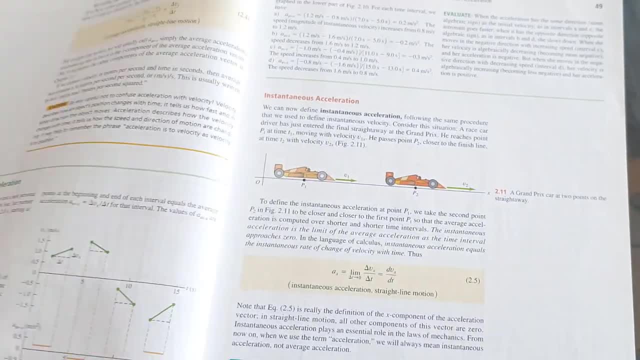 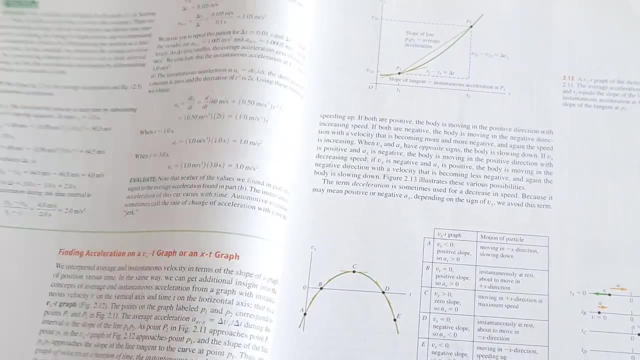 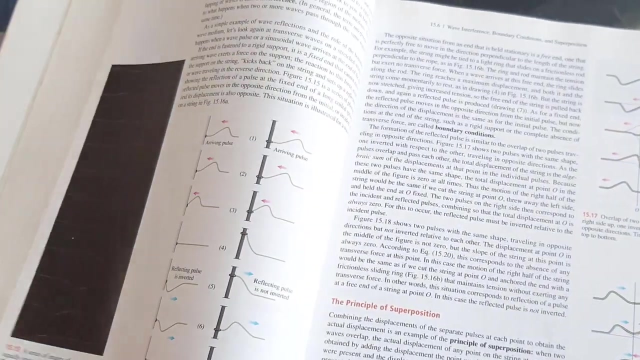 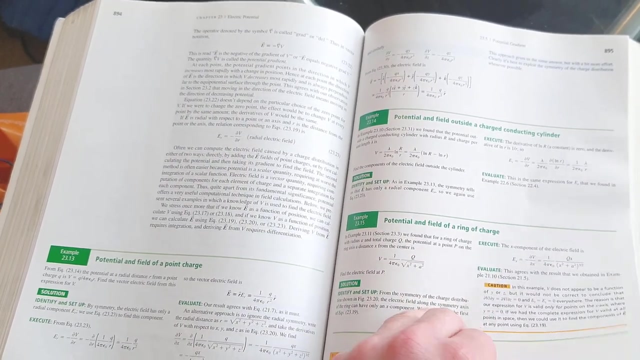 answer to this is Jung and Friedman University Physics. What I really like about this book is that it starts from the very basics, such as vectors, goes through all of kinematics, dynamics and classical mechanics on to electromagnetism, goes through the very basics, starting from Coulomb's law, all the way to the derivation of Maxwell's equations. By the way, this is: 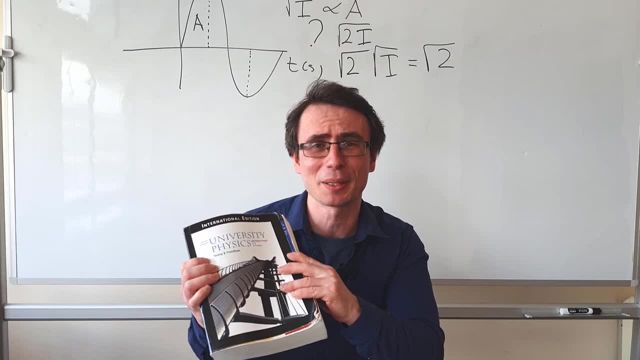 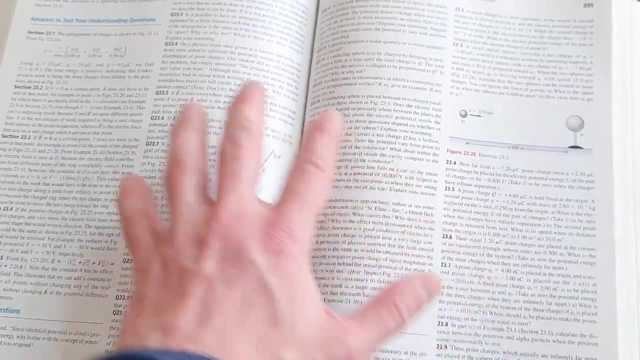 not a sponsored video in any way. this is actually my own copy that I bought from when I was a student. What I really like about this book, though, is that it contains an absolute wealth of problems, and you can really make sure that you've mastered the topics by checking in. 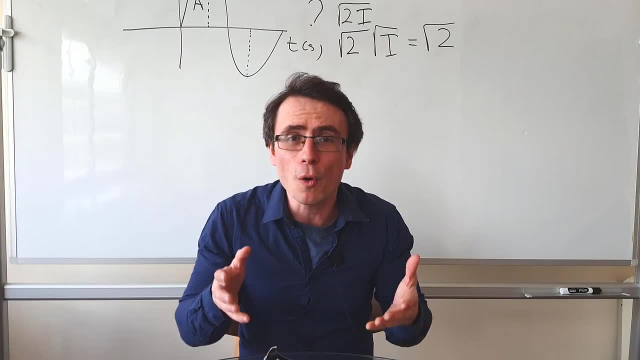 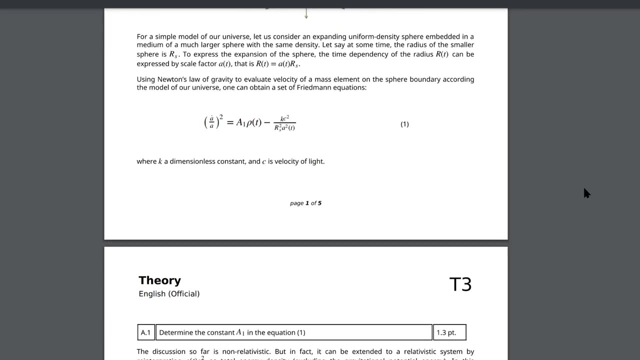 with the numerical answers at the end of the book. I've also noticed that some of the problems keep appearing in Olympiads and they're very, very similar to the GE Advanced as well. and have a look at this example in which I derived the second of the Friedman equations, which is included in 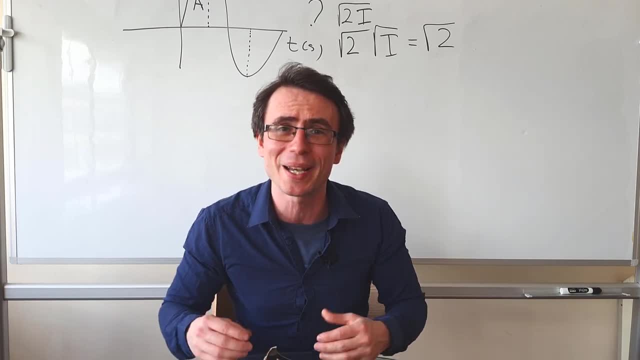 this book, but it also came up in the International Physics Olympiad, and this video is just over here. 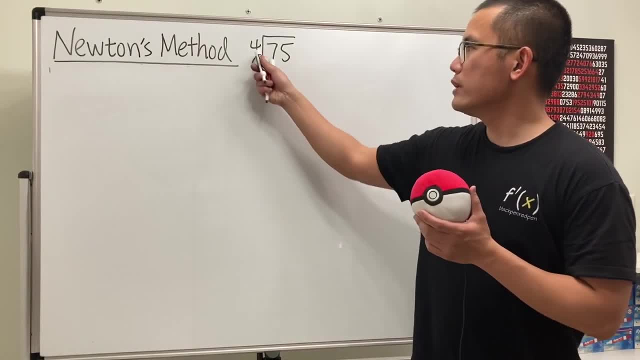 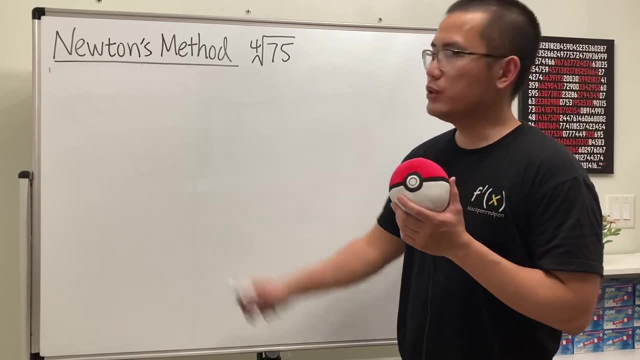 Okay, we'll see how to use Newton's method to approximate force root of 75.. And the first thing that we need is the function that we. Okay, we'll see how we can use Newton's method to approximate force root of 75.. 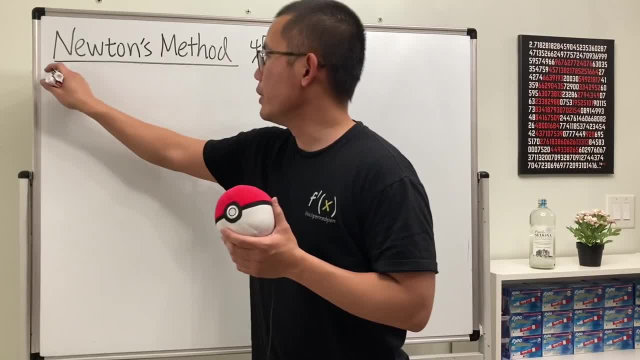 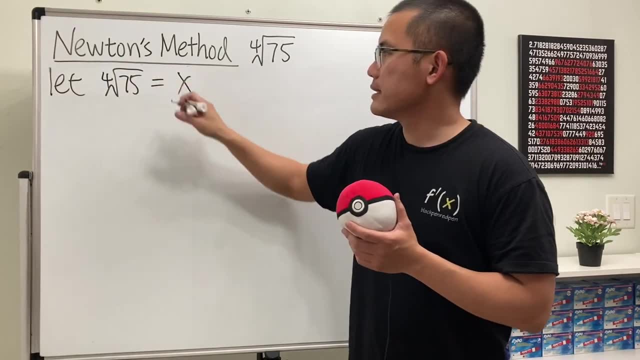 And the first thing that we need is a function, And this is how we can do it. We can code this to be x first, So the force root of 75, put that to be x, And then from here we can just raise both sides to the force power. 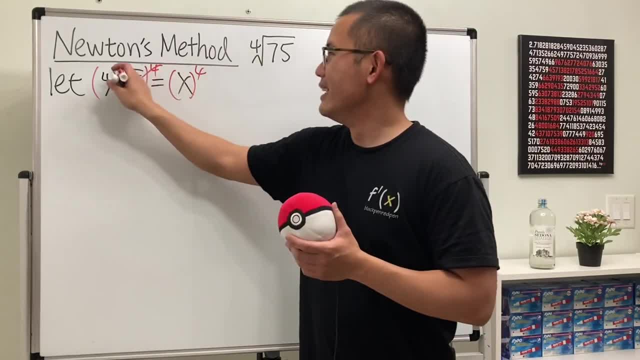 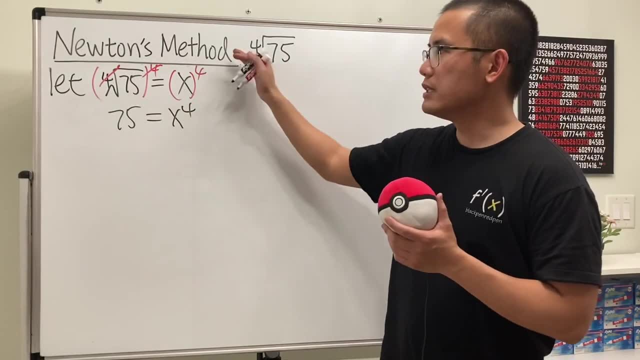 so that we can get rid of the force root And we get 75 is equal to x to the force power. And remember the purpose of Newton's method is to solve for the zero or the root of the function. So we want to see zero on one side.